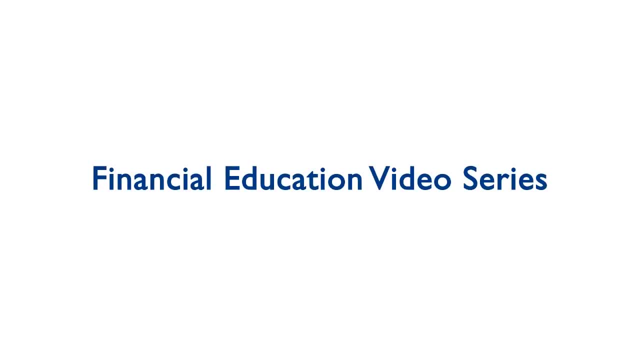 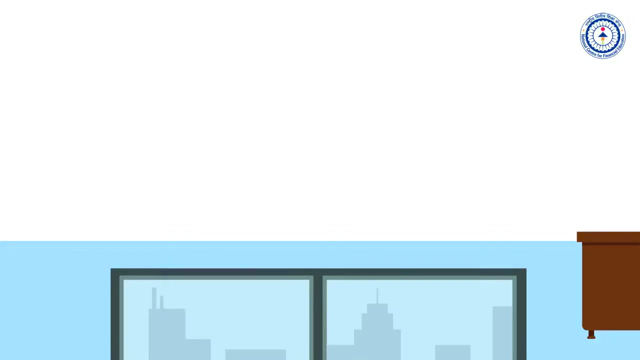 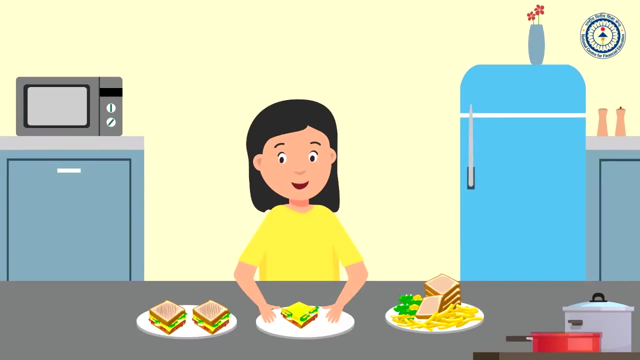 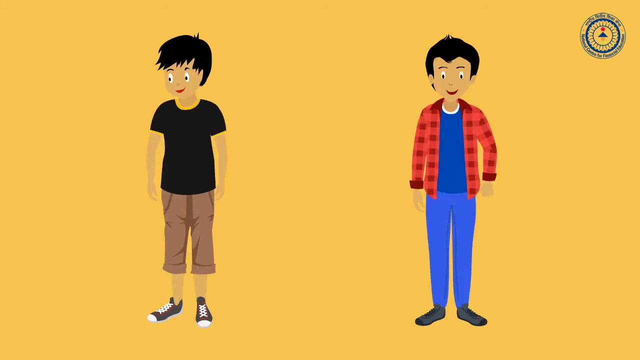 Saving Every coin counts. While our parents work hard to provide for our needs and wants, wouldn't it be nice to be able to help them in our own little way? Here is a story of two 11-year-old twin brothers, Naveen and Praveen. 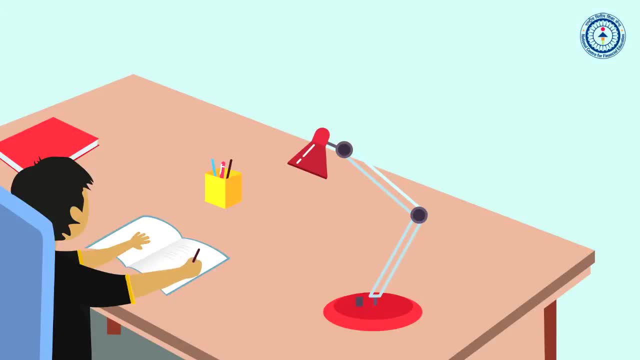 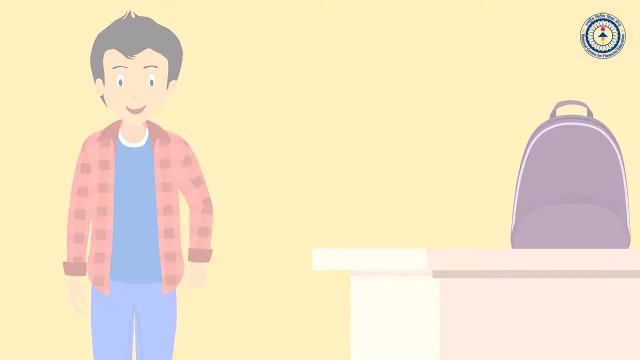 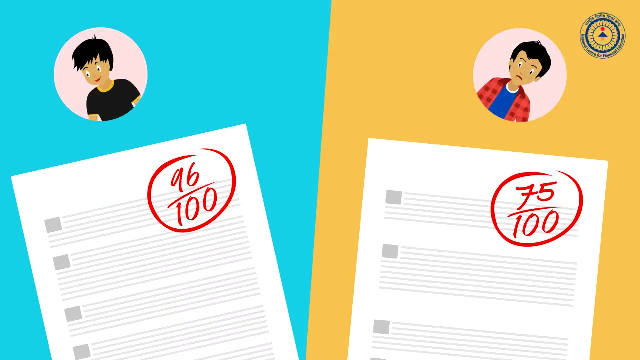 Naveen ensures that he finishes his homework and studies every day before going to play with his friends. Praveen postpones studying every day and plays all the time. While Naveen excels in his exams, Praveen gets an average score. 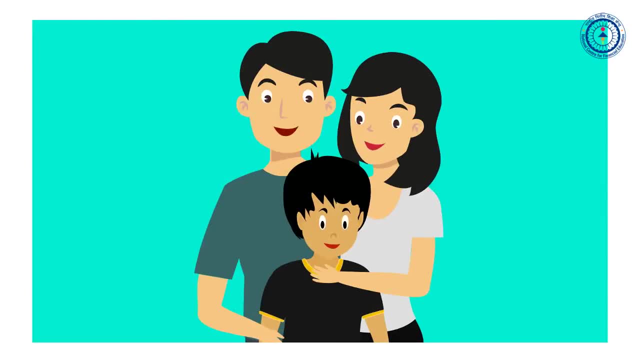 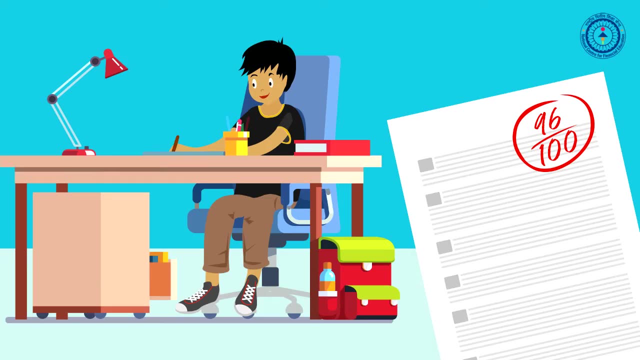 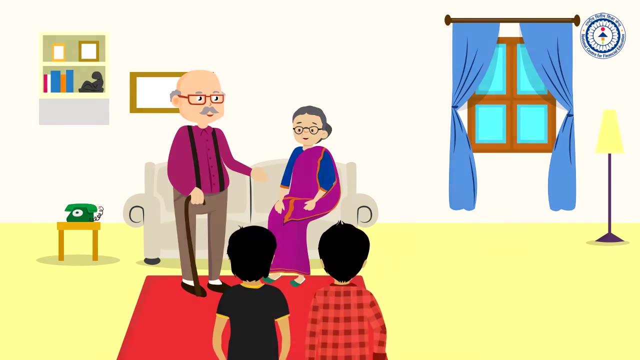 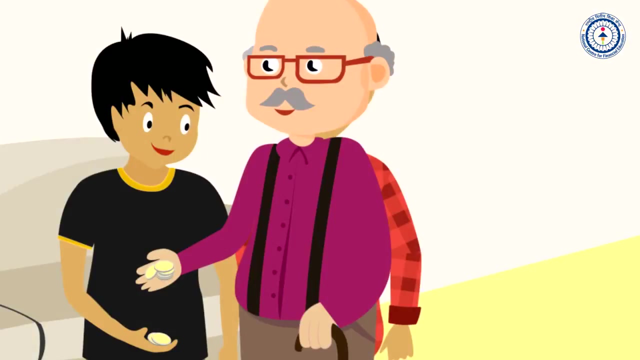 Naveen makes his parents proud and happy. This teaches us that regular practice can help achieve success. Now, every week, Naveen and Praveen would visit their grandparents' house. They would wait excitedly for the moment when their grandfather would give them a few coins each to buy whatever they wished to. 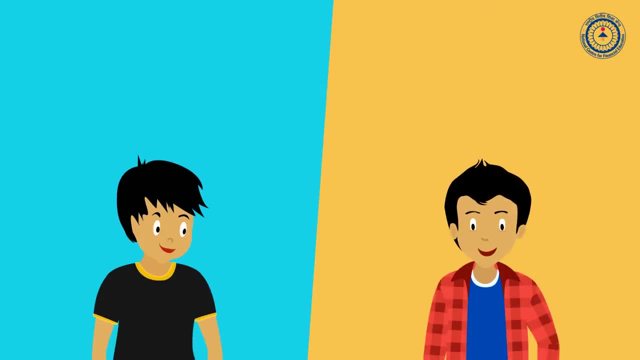 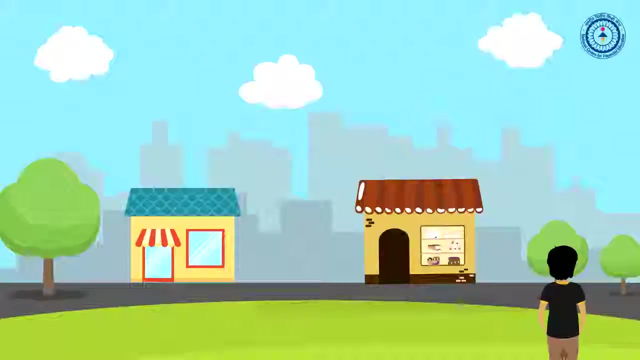 Both Naveen and Praveen liked different things. Naveen loved chocolates. Praveen, on the other hand, loved sports, especially badminton. Every week after the visit to the grandparents, Naveen would go excitedly to the local shop and buy chocolates. 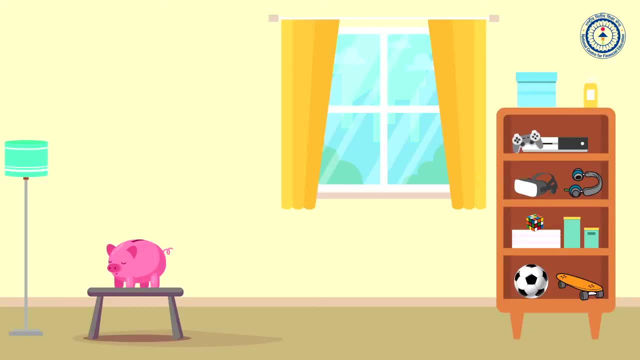 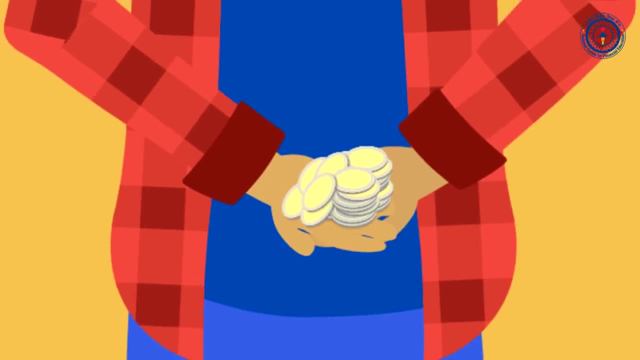 Praveen spent some of his money on candy but saved a larger part in a piggy bank. After a year he had enough saved to buy what he had wanted for a long time. Guess what he bought? A good quality badminton racket. 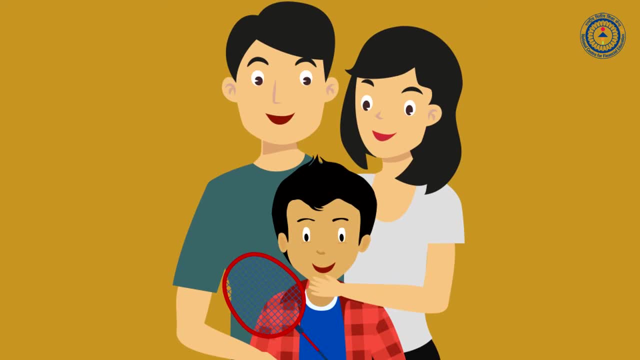 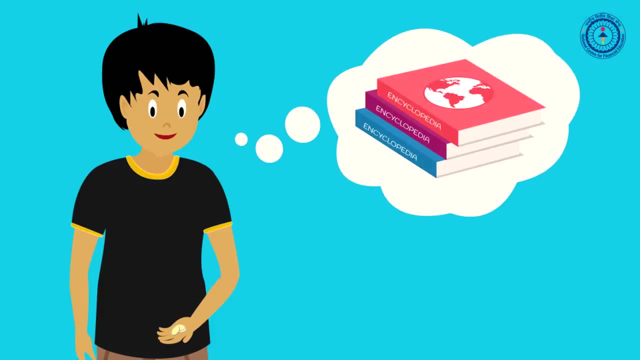 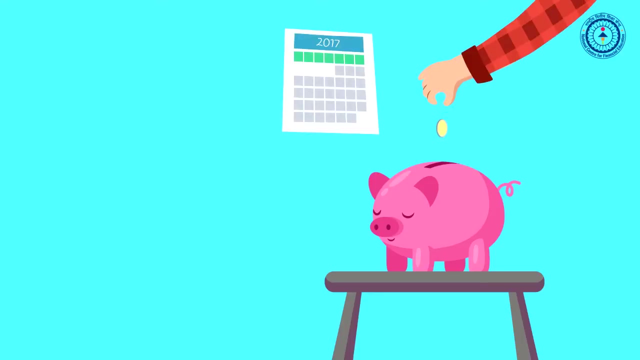 It was Praveen's turn to make his parents proud and happy that he bought this with his own money. Meanwhile, Naveen wanted an encyclopedia, but did not have enough saved for it. The moral of the story is, by saving regularly, a big or a small goal can be achieved.